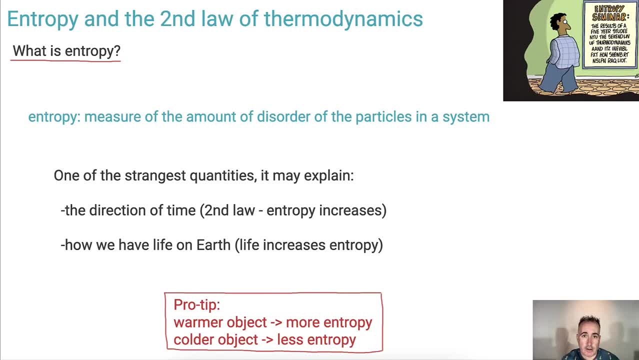 In this video we're going to be talking about entropy and the second law of thermodynamics. Now, what's important to understand for entropy is this right here: It's the measure of the amount of disorder of the particles in a system. So I like this one right here: entropy seminars. 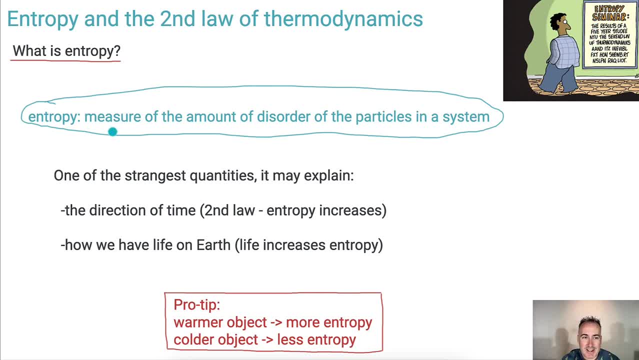 because things just get worse, because they're more disordered. But what I like about it is: well, it's very strange first of all, but it might actually explain the direction of time because it's irreversible. So it's going to explain a little bit about the second law that. 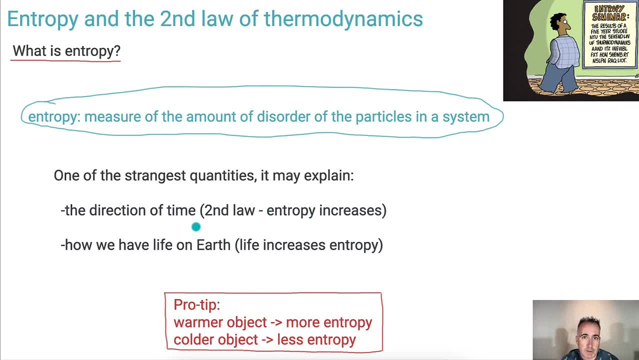 entropy increases. We'll see that later, But also it might even explain what life actually does. So we actually increase the entropy. So a nice pro tip here: just remember this that warmer objects have more entropy because, remember, there's more sort of random motion in warm things than there. 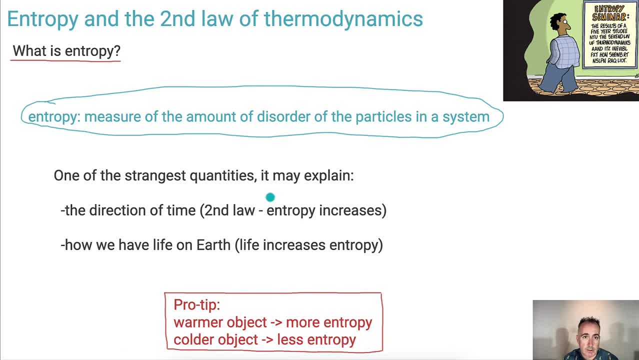 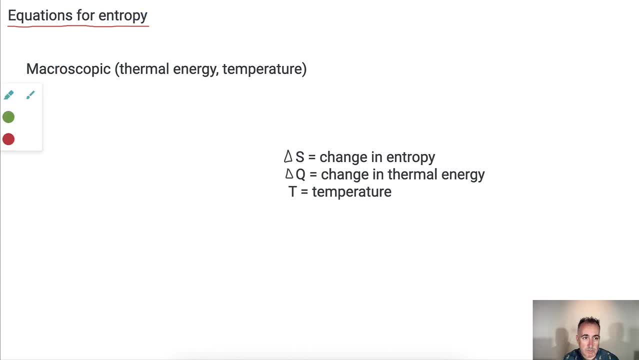 are in cold things, So this also has to do with temperature as well. So let's look at this equation actually. So we have these equations for entropy themselves, So we have macroscopic, which means for sort of larger objects, things like thermal energy and temperature. 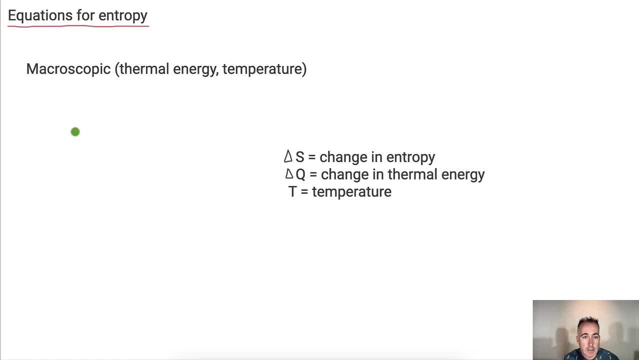 we'll be comparing that to, for example, microscopic in a second here. So first of all, we have this equation right here. It goes like this: the delta S, so the change in entropy in a system is equal to the change in thermal energy divided by the temperature. So this: 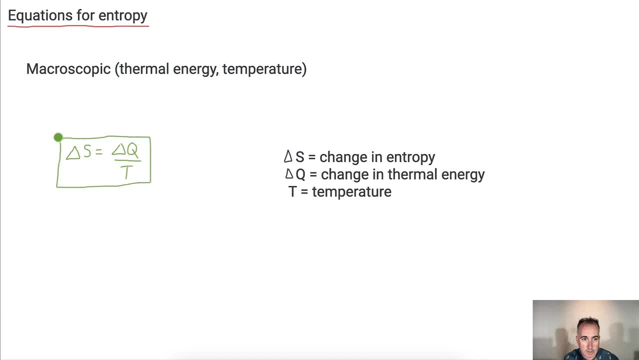 is in your data booklet. hooray, But there we go. So what are the units? Well, change in entropy- We'll have to look at this in a second here. So change in thermal energy is in joules. Temperature should be in kelvin. So does it make sense what the units for? 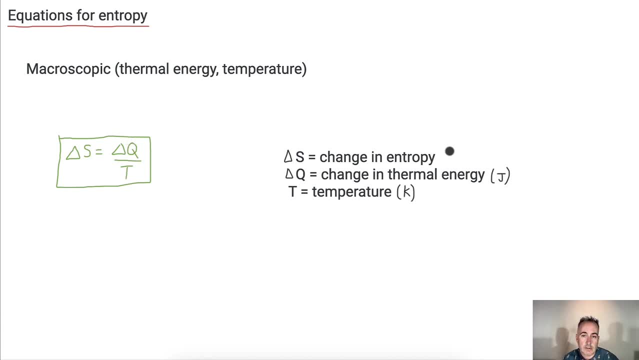 entropy then Should be in joules per kelvin, So you don't have to memorize all the units. Sometimes you just figure them out based on the formula. So hooray. Now let's look at this one right here for microscopic. So instead of being a delta S like before this, 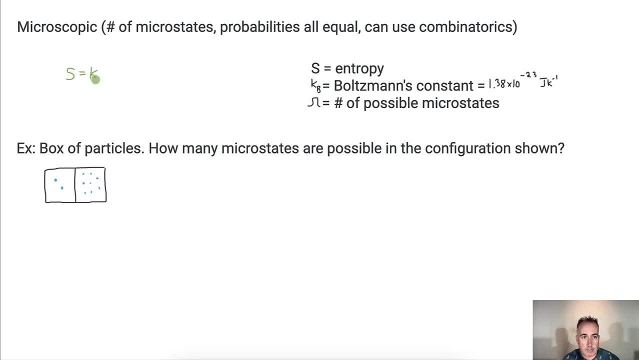 one's just equal to S. So let's say entropy equals and it's just Boltzmann's constant. yet again, this time times the natural log of this ohm here, or this omega. So this is times the natural log. So what do we? 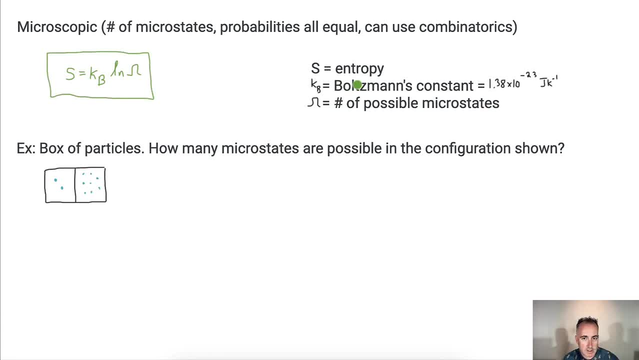 do about this here? What does this mean? Well, first of all, hopefully you understand this Boltzmann's constant. That's at least one you've seen before: Entropy. well, entropy is going to be in again, joules. 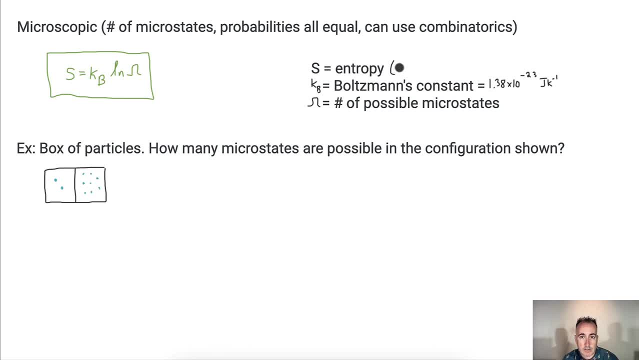 per Kelvin, So we can write that one down at least. So that's in joules per Kelvin And this omega is the number of possible microstates. I'm going to explain this now. So let's just say we have a box of particles here, So we have a bunch of different particles. They're 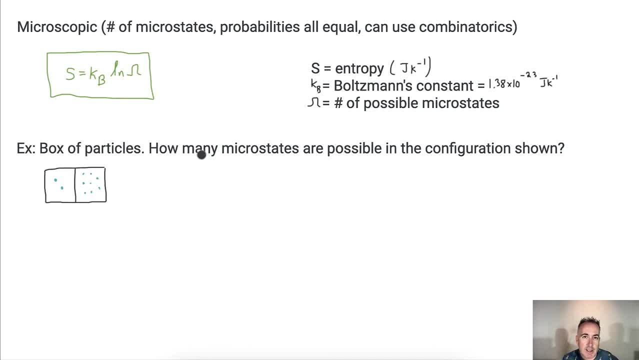 equally likely to be on the left side and on the right side. We're basically looking at how many different ways are there to arrange the particles in this way, In other words, when there's two on the left side and let's see there should be eight on the right. 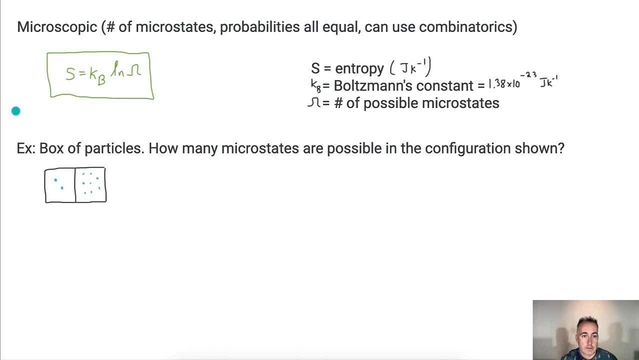 side. So how many different ways are there of like lining them up? So there are, for example, 10 ways to organize this first one right here, to get this first one over there. So we'll do 10.. But then of course there's 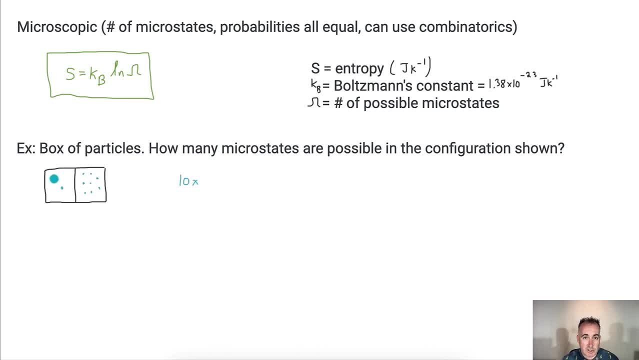 once this one here has been over there, the different ways of getting a second one over there. there's only nine ways of doing that. So that should be. you'd think it should be 90. But I'm going to write this down right here. But those 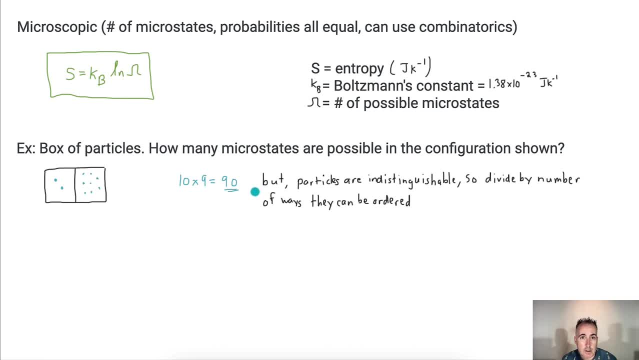 particles are indistinguishable, So we have to divide by the number of ways that you can order them. So in other words, in this case, of here two. So that means I'm going to take my 90,, divide that by two and I end up with 45. So the number of microstates. 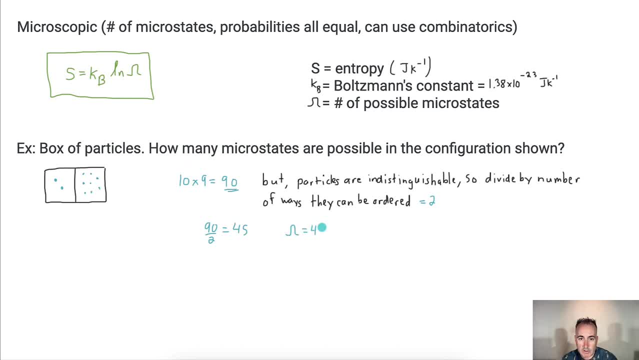 then I can say that this omega then equals 45. So that's how I would, for example, solve this one. Now there's another way of doing it. You could, depending on which math class you're taking, and if you've learned about this, you can use combinatorics. So this is something for 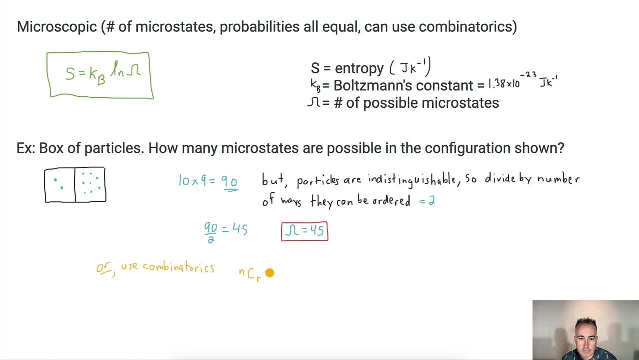 example called, for example, NCR, for example. So if you remember ever doing that stuff and if you've never learned it, don't worry, then just use this method up here. But otherwise I just want to show you how this. 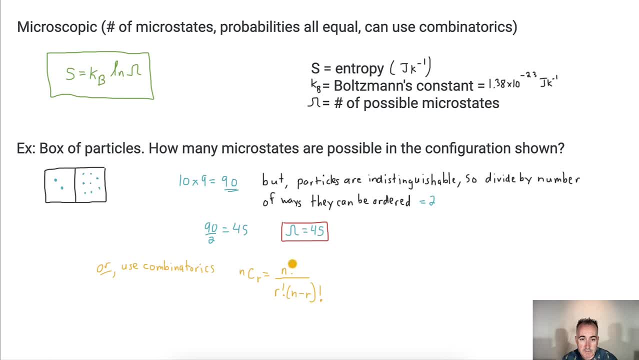 actually relates to, for example, NCR. These are factorials, by the way. So in this case, right here, then in this case right here, we would have 10C2, because we're looking at how many different ways are there of organizing, how many different combinations. 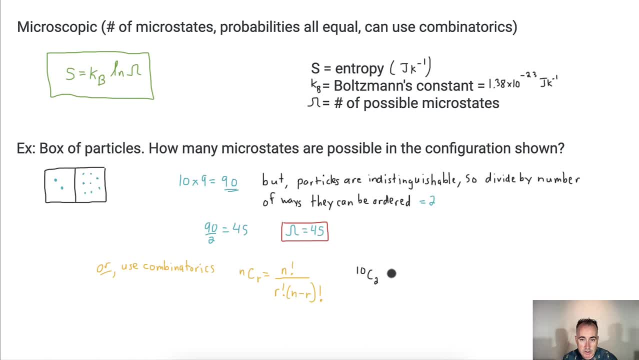 are there of organizing two from 10.. So in this case, right here, we would say: well, first of all, it's 10 factorial, So that's 10 times 9 times 8 times 7 times 6.. This gets a little bit boring. 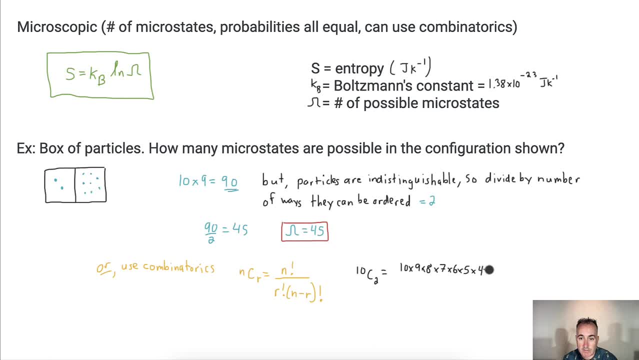 Once you've done it a lot, you skip all these steps right here. but it's okay. I just want to show you everything. Times 2 times 1.. All that is divided by, let's see R, factorial, which is 2 times 1.. That's what a factorial is, All that times. 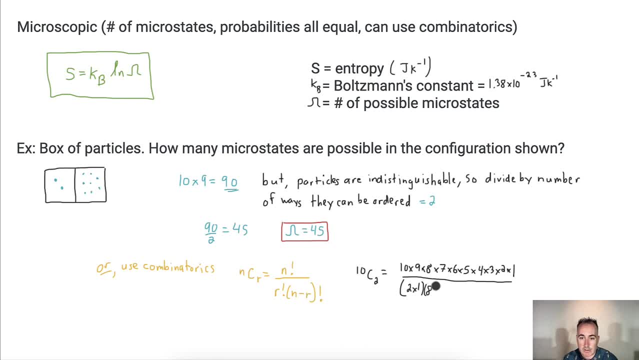 N minus R. Well, that's 10 minus 2, so that's 8 factorial. So 8 times 7 times 6 times 7.. 5 times 4 times 3 times 2 times 1.. And what's nice about these factorials? what happens? 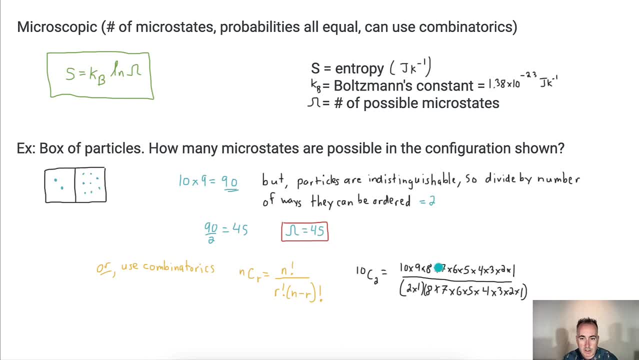 then if you've experienced these before, you'll see that, hey, look at that. The 8, 7, 6, 5, 4, 3, 2, 1 cancels out this one right here, which is nice. So you have 10. 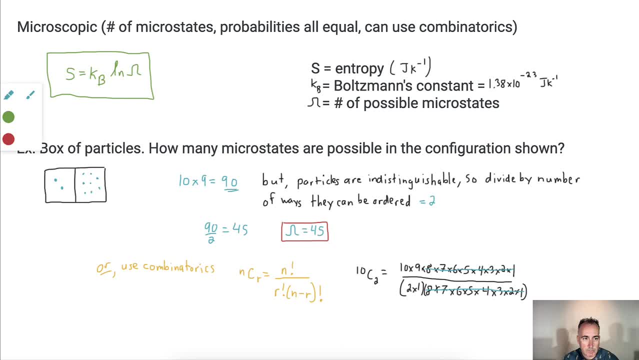 times 9, divided by 2.. So, do you see, you end up with the same thing right here. You end up with, well, 10 times 9, divided by 2, which is 90 over 2,, which is 45.. 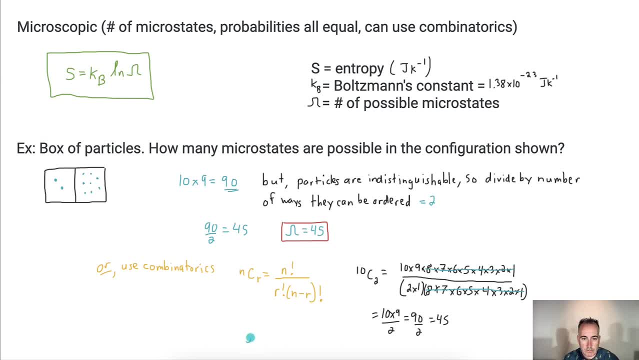 So it still works. So just to show you now, if you don't know this method right here, no worries, You don't have to worry about this. And for example, this bottom one here is combinatorics method, because you're not given this formula on your physics exam. This 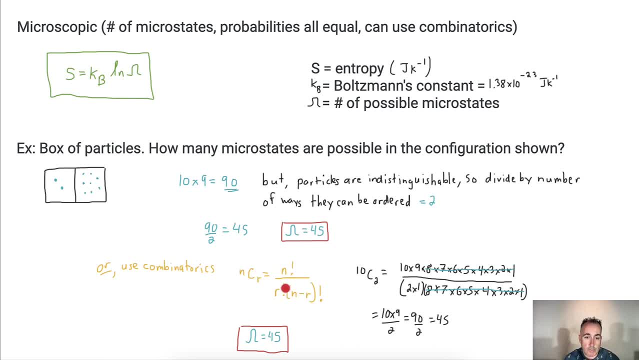 is actually for your math ones, if you have it. But I'm just trying to make the link at least to combinatorics, in case in your math class you've learned it. Otherwise, you just have to think kind of carefully about how many different ways are there of arranging. 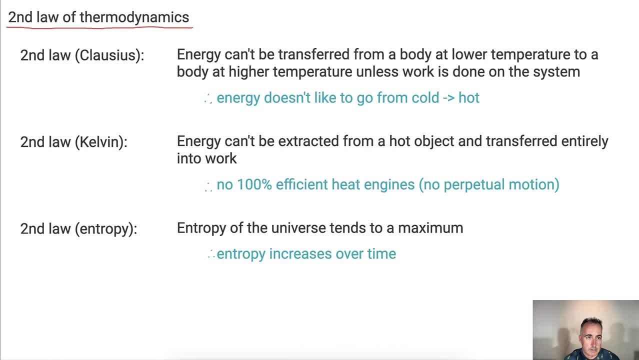 these, for example, 2 from 10.. So let's talk about now the second law of thermodynamics, And there's a few different formulations. There's the Clausius version, the Kelvin version and we'll do the entropy. 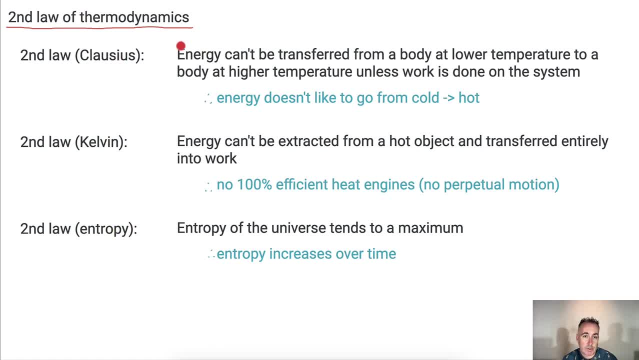 version as well. So the second law really is all about. well, energy can't be transferred from a lower temperature to a higher temperature unless work is done on the system. What it really means is just: energy doesn't like to go from cold to hot, For example, if I had 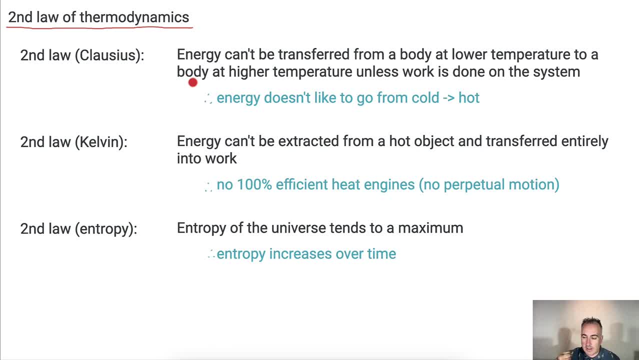 you know, a cup of hot chocolate, for example, in my hand and I'm sitting in a room. there's no way the hot chocolate's going to get in there, So I'm going to have to do a little bit even hotter, for example, Like the hot chocolate's going to get colder, right? Because 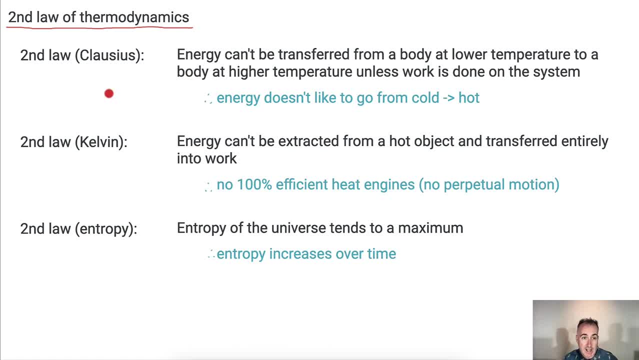 it's going to go from, you know, hot to cold- The Kelvin version of it, for example. second law is that energy can't be extracted from a hot object and transferred entirely into work. What it really means is that there's no such thing as a heat engine. then it's. 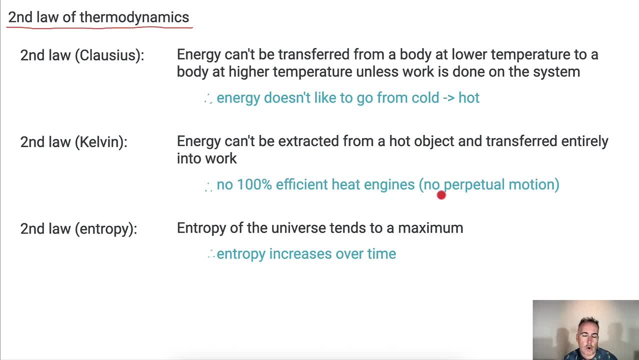 100% efficient. So, for example, you can't have perpetual motion. There's always some losses due to friction and other things. And finally the entropy version, and I think this one right here is my favorite version, at least as it relates to entropy, of course. 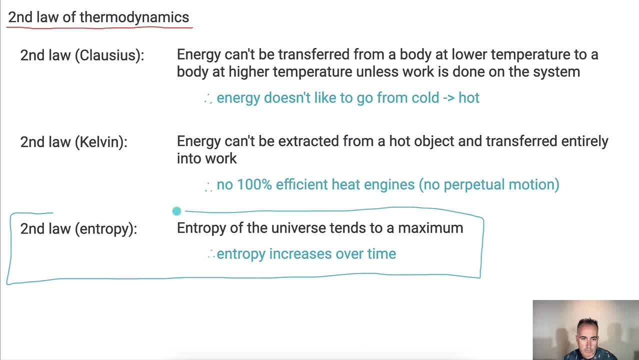 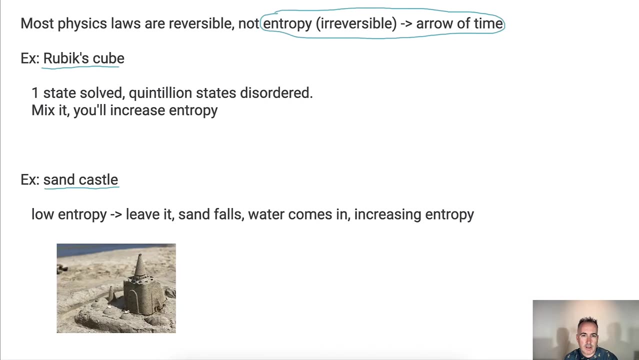 is this one right here. The entropy increases over time overall. So that means on a grand scale, the entropy of the universe goes up, The amount of disorder goes up, You know, the energy, for example, of the universe spreads out. Now, does that mean that you always have to have that happen? 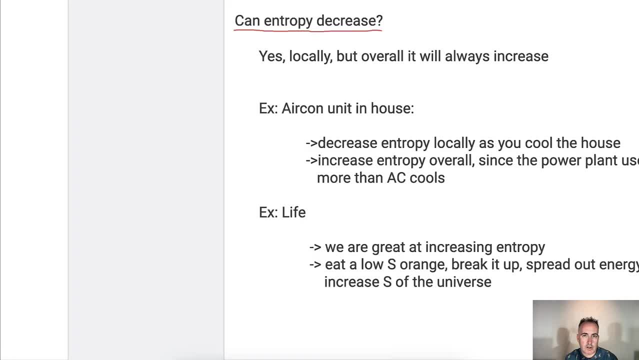 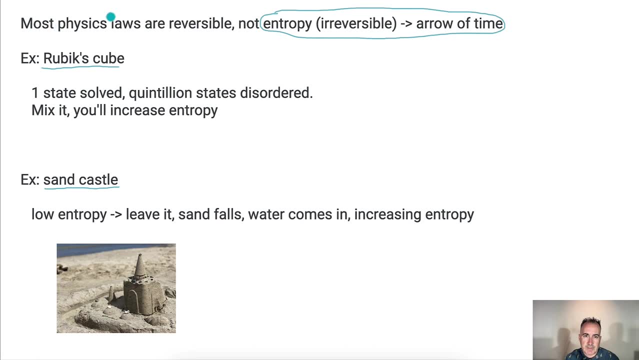 No, no, no. Sometimes you can have- for example, over here you can have- entropy decreasing. Sure, I'll explain that later. but we can go a little bit deeper here. Entropy: remember I talked about before How it's related to the arrow of time. Well, that's because entropy is not reversible. 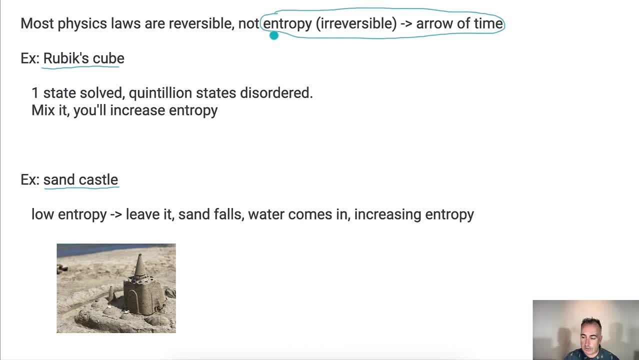 Most processes in physics are reversible. You know, if I do something one way, I can reverse it and do it the other way. But entropy, no, It seems like it's a one-directional thing And because of that a lot of people, at least within physics, like to tie entropy to the 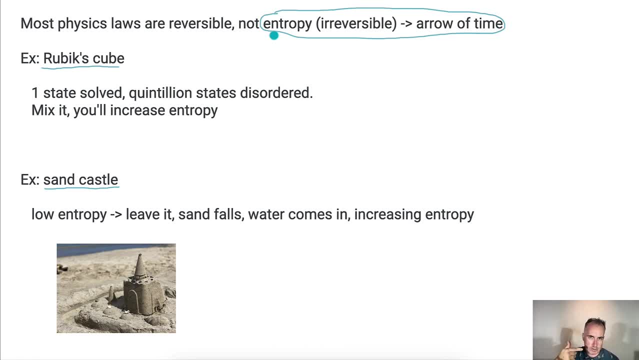 direction of time, because time also seems to be something that we can't reverse. So we think that entropy, which is irreversible, might very well be related to the sort of direction of time. And another way to just sort of try to think about entropy is over time, lots of you know. 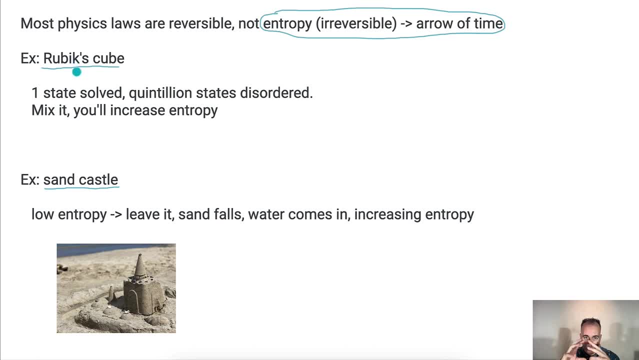 lots of different examples, but I'll just think about a Rubik's cube. If you've ever seen those little cubes, you just spin them around. I mean there's only one way to have it solved, but there's, you know, billions and billions and billions of ways for it to. 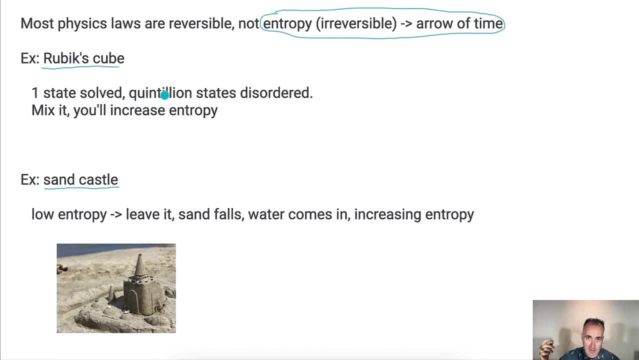 be not solved. So clearly it's: the more you turn it, the more you increase the entropy. Same thing with, like a sandcastle. I took this picture actually, as my daughter built a sandcastle last year, for example, So I took a picture of it. But I was just thinking.